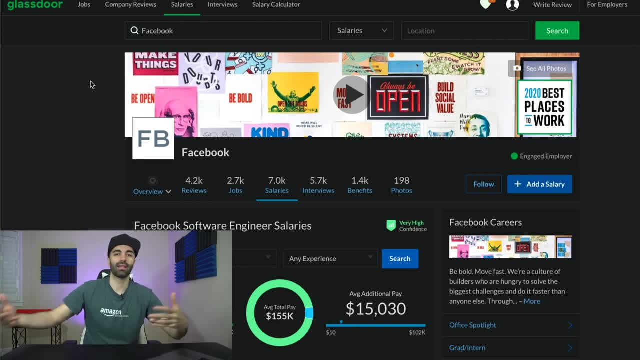 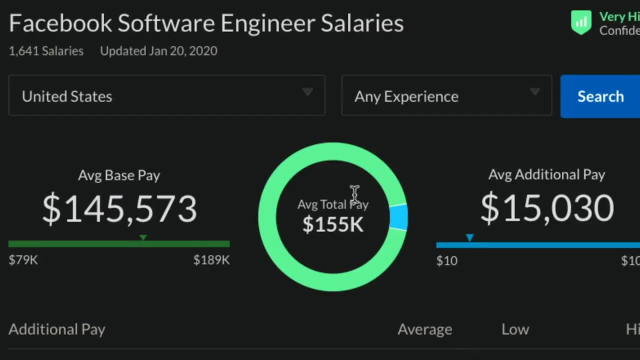 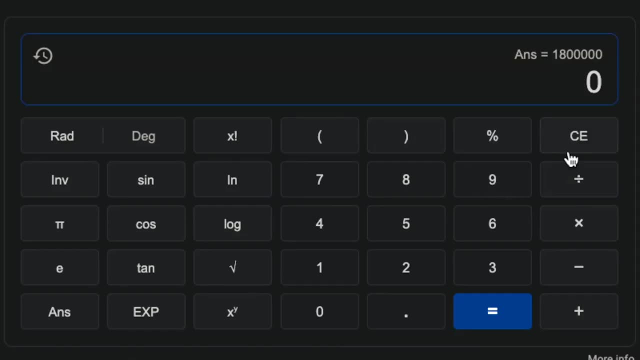 let's look at what the salaries are like. So say, we work at a company like Facebook. if we go over to Glassdoor we see that the salaries here are about 155,000 total for a Facebook engineer. So let's just say 150,000.. So if we go over to our calculator and we say, okay, we're making $150,000. 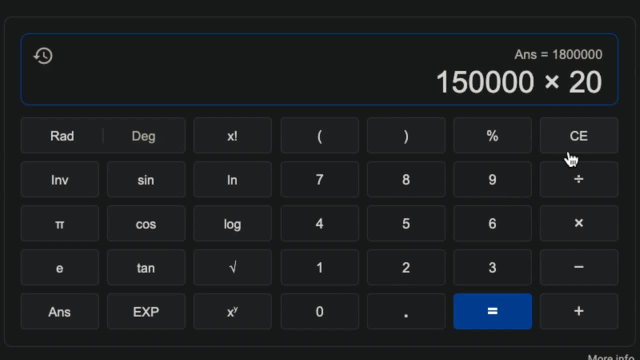 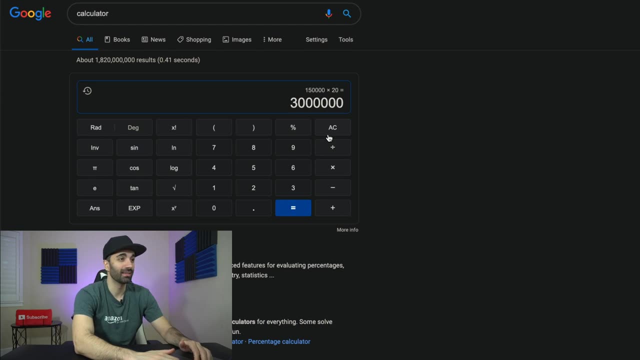 and we're making that for 20 years. right, that's going to give us 3 million dollars, Cool. So one thing we need to take into account are taxes. Unfortunately, they take a lot of them out, and especially here in California, I think it's about a third for taxes. 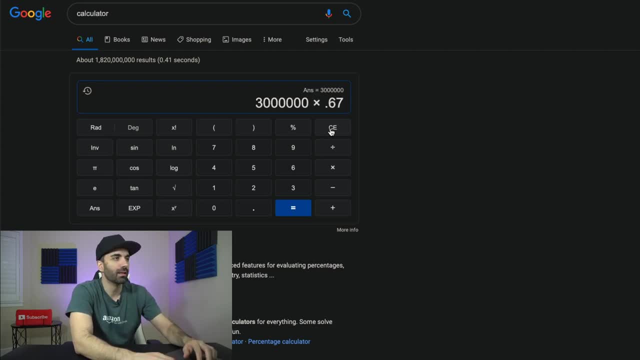 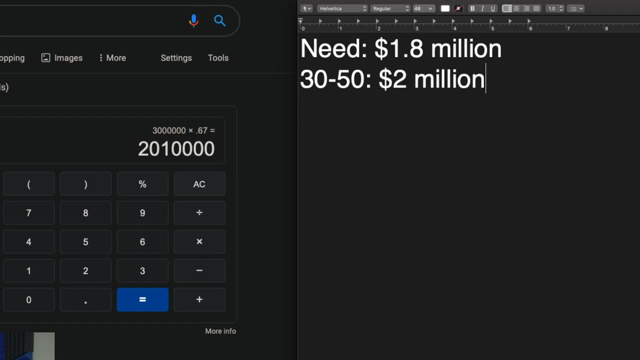 so let's say: you know, one-third of three million dollars is a million, so we're gonna be left with about two million dollars, which is still not bad right? so basically, from 30 to 50, we made two million dollars. congratulations. Now one thing you might be saying is: okay, yeah, it's really not that. 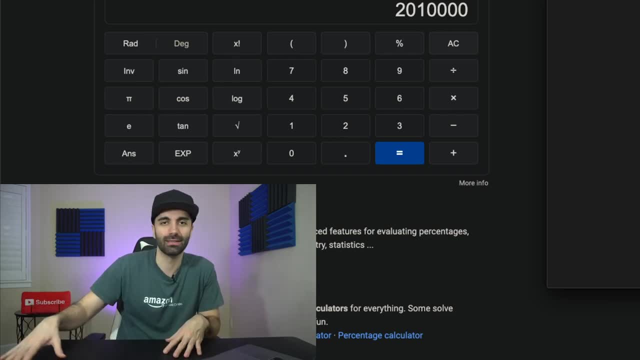 bad. but to be honest, first of all, retiring early isn't gonna be easy, otherwise everyone would do it. so I mean there has to be some challenges here, and really 150, for you know, say, by the time you're 30, if you're coming out of school, you're gonna have like eight years of experience, and we're also 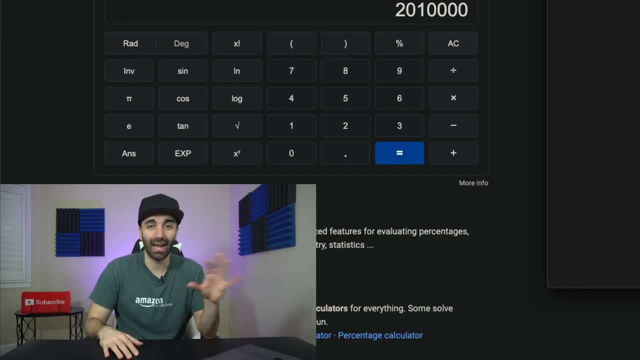 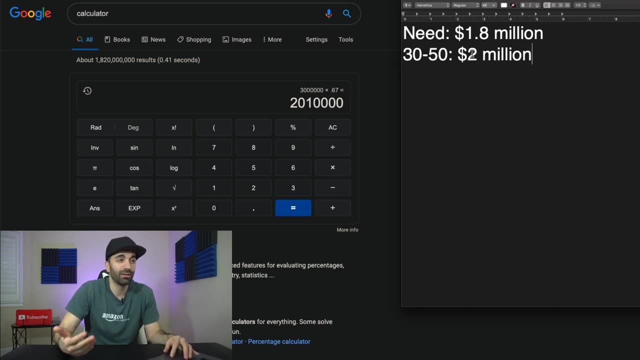 assuming that you're not getting any raises here. so I think like an average of 150 is very realistic. Now, one thing that we didn't take into account is: okay, at 50 we're gonna have made two million dollars. however, from 30 to 50, we're gonna have to make two million dollars, So we're gonna have to. 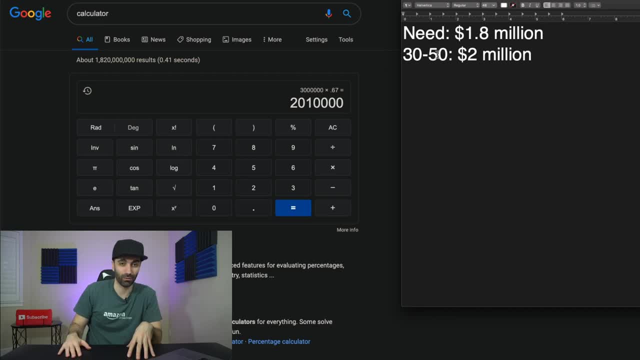 spend money throughout that time, right? so that's something that we haven't accounted for yet. So let's go ahead and figure that out. So we need to figure out what our monthly expenses are. So let's say, rent here in the bay area is about you know if you get your one bedroom apartment. 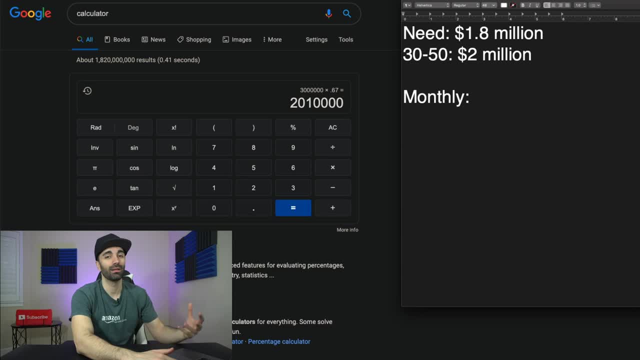 it's gonna be about three to even four thousand dollars. Let's say we want to be a little frugal and we get a roommate, so with rent and utilities we're paying about fifteen hundred dollars. We're gonna spend another thousand dollars on food. We're gonna say: you know, 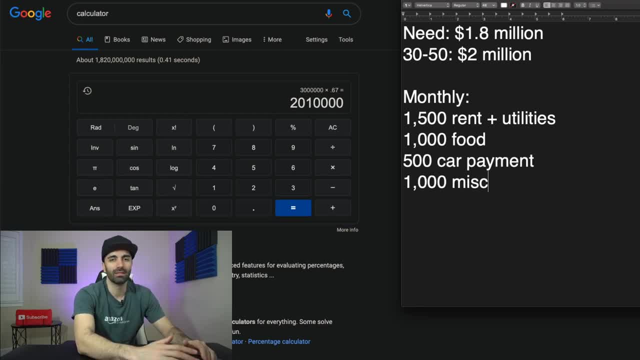 we're gonna spend another thousand dollars on food. We're gonna spend another thousand dollars on food. maybe you have a 500 amount car payment and then let's just say we have a thousand dollars for just anything miscellaneous. so this comes out to four thousand dollars a month. so if we say four, 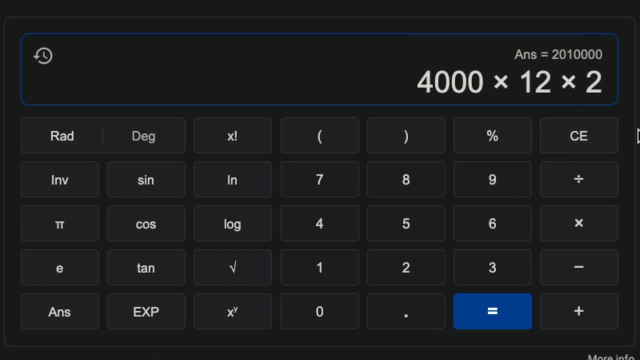 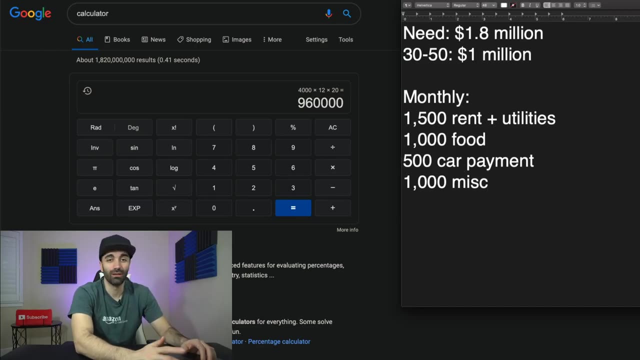 thousand dollars times 12 months, times 20 years. well, we just spent a million dollars. so if we go back here from this 30 to 50, we're gonna have one million dollars to show for it. so now we're short eight hundred thousand dollars. but not to worry, we're gonna fix this. if we go down a monthly, we're 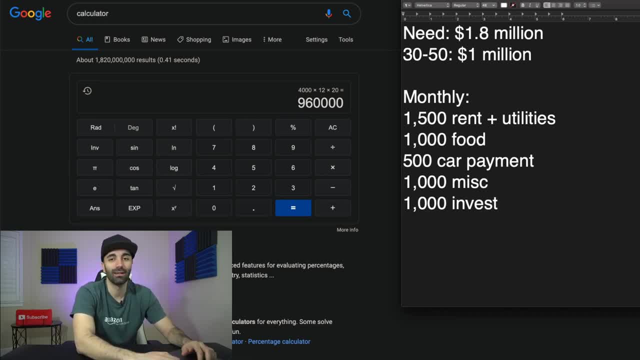 gonna spend an extra thousand dollars and we're gonna just put that in investments. so now we're gonna be spending five thousand dollars a month, which now puts us at 1.2 million dollars. so right now we're actually short a million dollars. so how are we going to make up a million dollars? 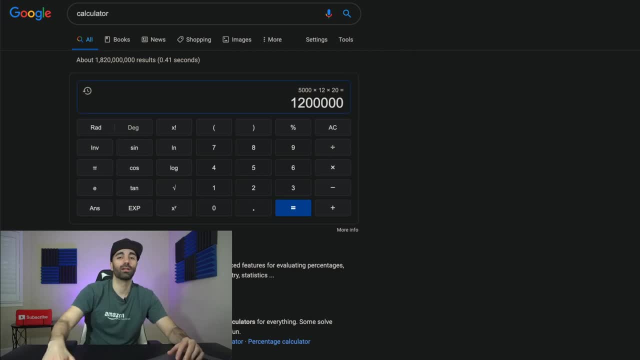 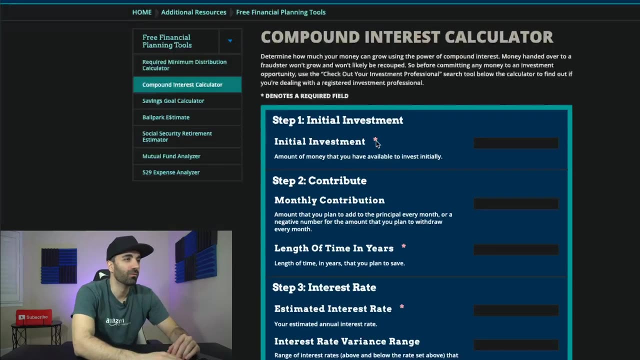 well, since we are investing this, let's go over to figure out how much we can make investing a thousand dollars a month. so if we go to this website here that has a compound interest calculator, we need to figure out what our initial investment is. so there's this other website here. 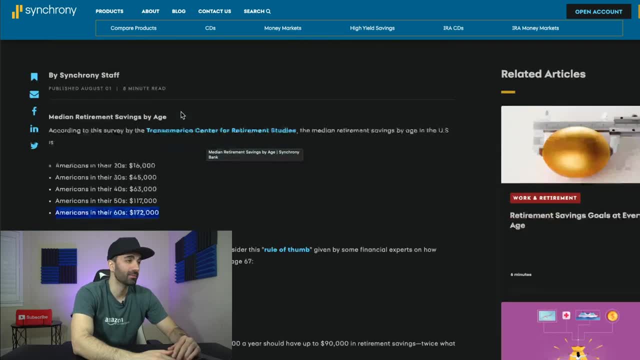 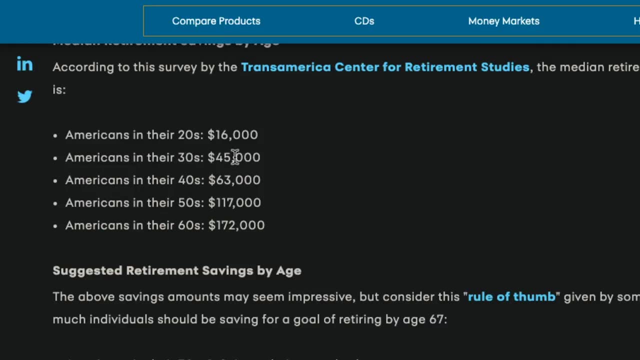 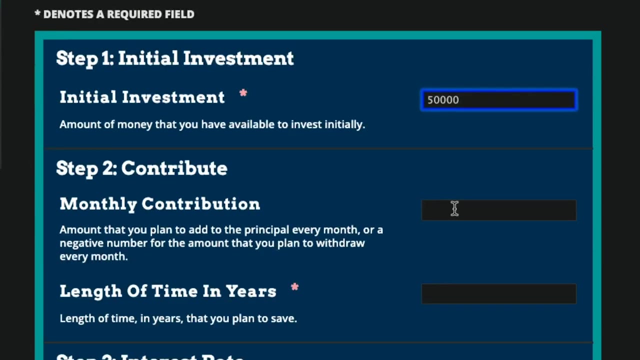 that's calculates the median retirement savings by age. so if we go down here, we see that for someone who's in their 30s they're going to have about 45 000. so let's just round that up to 50 000.. so if we go here, we have fifty thousand dollars. our monthly contribution is a thousand dollars. 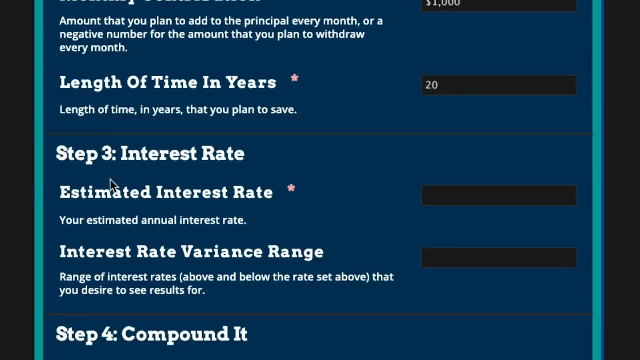 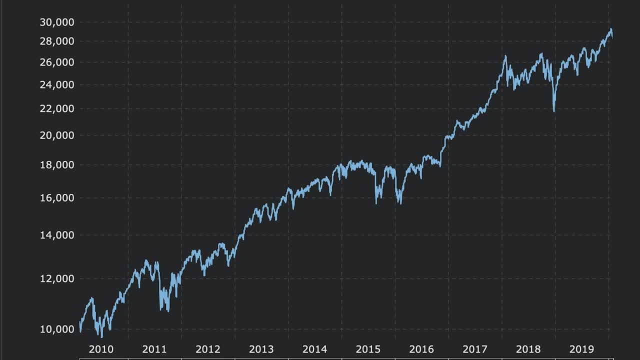 the length of years is going to be 20 years and now we need an estimated interest rate. so if we go over to this website here and we look at the 10-year chart of the dow jones, which is pretty much what tracks the entire stock market, um, if we go to the last 10 years, we see 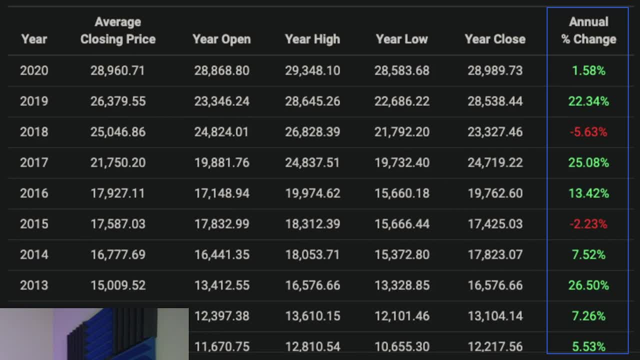 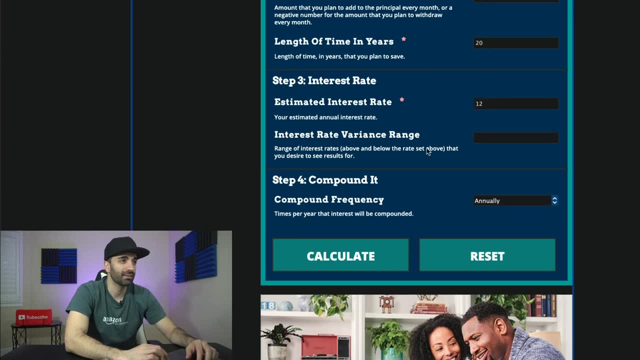 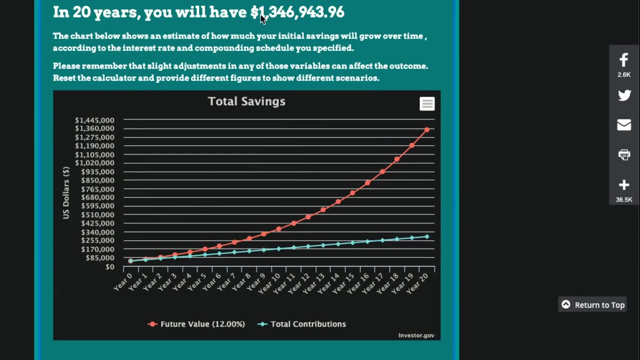 that i mean it fluctuates every year, but the expected average gains that you're going to get is about 12. so if we go over here and we say, okay, we're going to be getting 12 gains and that 12 gets compounded annually. so if we go ahead and calculate this, we see that we have. 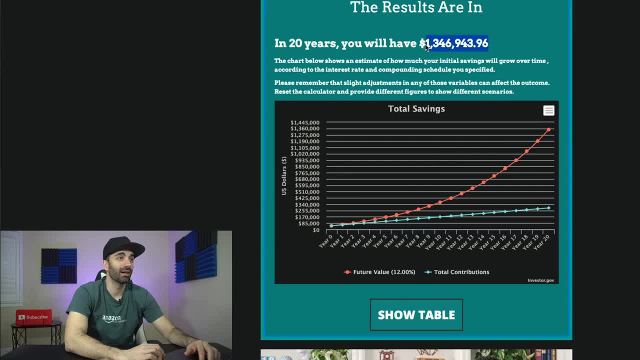 1.3 million dollars. so pretty good, right now, this- the money that you gain- will be taxed, which is about a million dollars. so we're gonna lose about three hundred thousand. so we're gonna make about a million dollars there, right, cool. so we have 1.8. right and now. 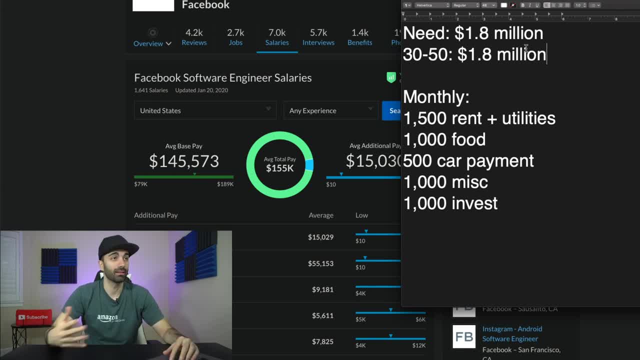 we have enough to retire now. another thing to mention that's a good thing is once you hit 50, you're not all of a sudden gonna take out your 1.8 million, right? this is still gonna sit and ride in your investments, so maybe from you. 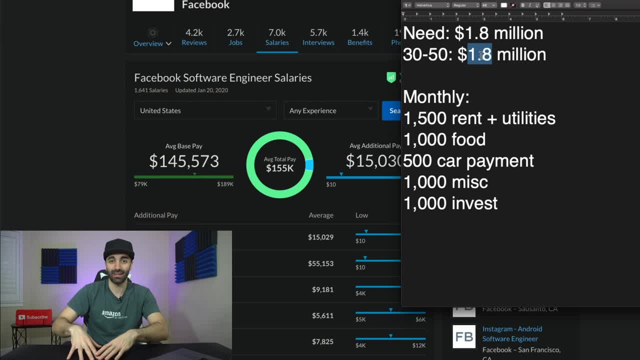 know, once you get 50, you're just gonna be taking out like five thousand dollars a month and the rest of that is just gonna be growing and growing. so not only do you have enough to retire at 50, you're actually gonna. your money is gonna grow exponentially throughout your retirement years. so what are some of the risks that we could run into here. well, first of all, the stock market could crash really at any time. right, we haven't had a real crash in about 12 years and, although you never know, it's pretty unrealistic to think that we're not gonna have a crash in the next 20 plus years. another thing is that you might get married and end up getting divorced and end up losing a lot of money there. the divorce rate is about 50%, so you never know. you might get married and end up getting divorced and end up losing a lot of money there. the divorce rate is about 50%, so you never know. and you might end up having several kids. the average cost of a child from zero to eighteen is about two hundred fifty thousand dollars. so if you have two kids that's half a million dollars right there. other things that aren't really risks, but our facts are, first of all, inflation. a million dollars today will 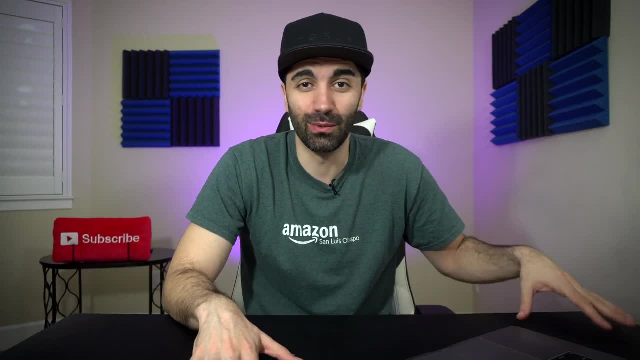 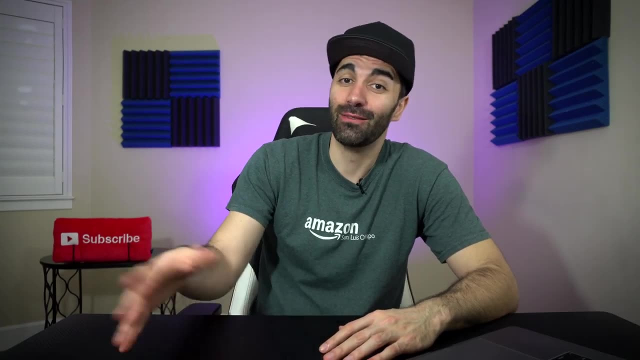 not be worth nearly as much in 20 years, just as 20 years ago a million dollars was worth a lot more. so these are definitely things that you have to take into account. one thing that could actually help you out is living at home. I know that in the United States it's kind of weird to live at home, but it in most other countries outside of the US. it's kind of weird to move away from home until you get married here in the US. if you know, say you're 30 years old and you're living at home. people might call you a loser, but to be honest I'd. 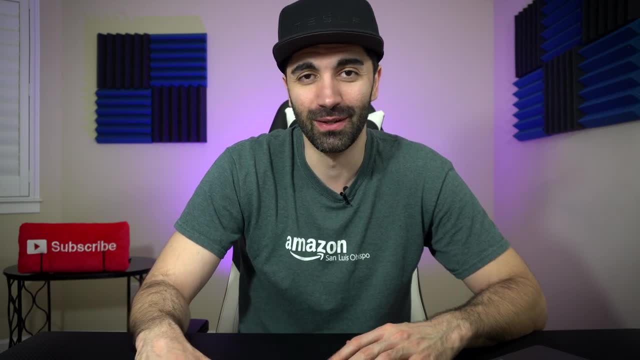 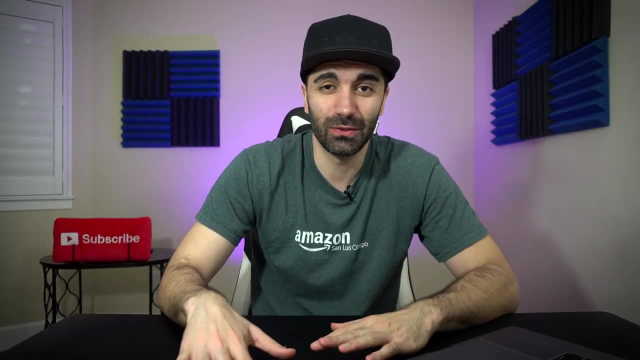 rather be a loser, with an extra three grand in my pocket every month. so I mean, if it's something that's possible for you, I would definitely recommend that you at least consider it. so in conclusion, is this really worth it? and in my opinion, it's not. to go this route means that you're probably gonna be. 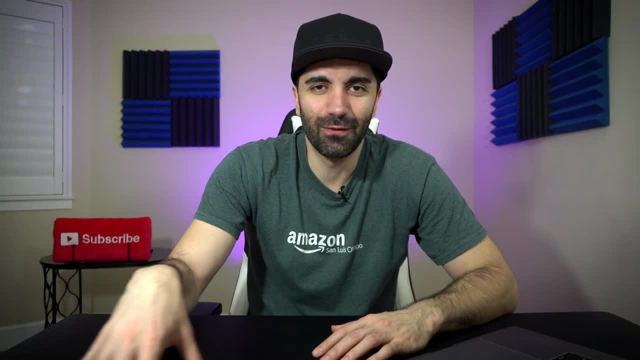 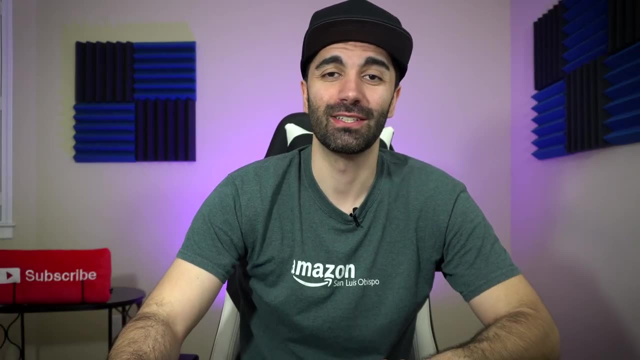 penny-pinching most of your life and it's just a very defensive strategy and I don't really think, even though you I mean it will be nice to retire early, you're not really living, you know. my recommendation is, you know, be a little bit more offensive, try and maybe start a 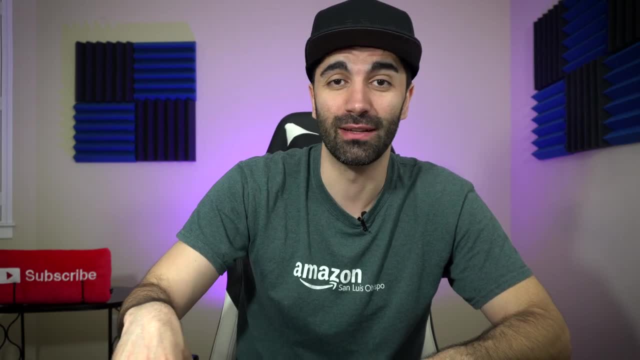 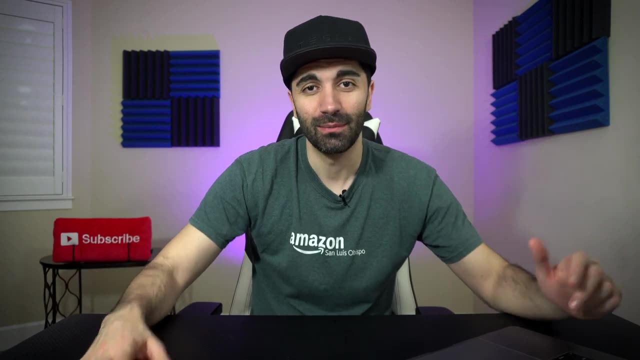 side hustle or start a business, maybe increase your income more rather than decrease your spending. but, as you saw in the video, if you do take the strategy that I just went over, it's definitely doable. so I mean, it's really just up to you guys, maybe. maybe you're fine, you remember, you're like, you know I'm a very 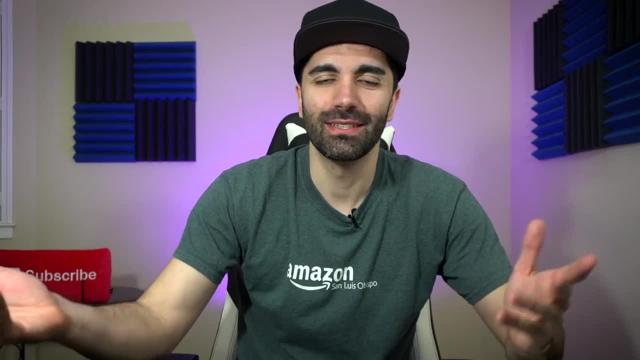 frugal person. I don't need to spend a lot of money, I'd rather just not work. I don't need to put that much of my money on selling stuff you like for real. and mostly you know this was just hypothetical, it was just for fun, just to. 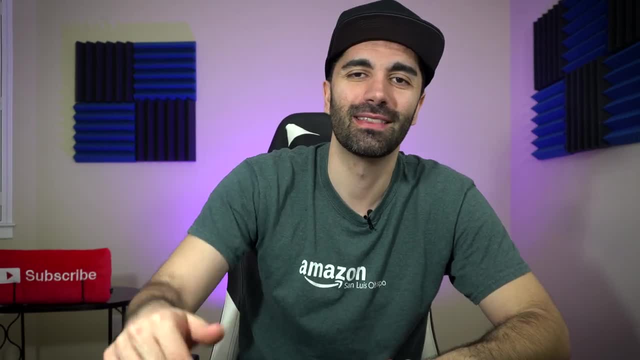 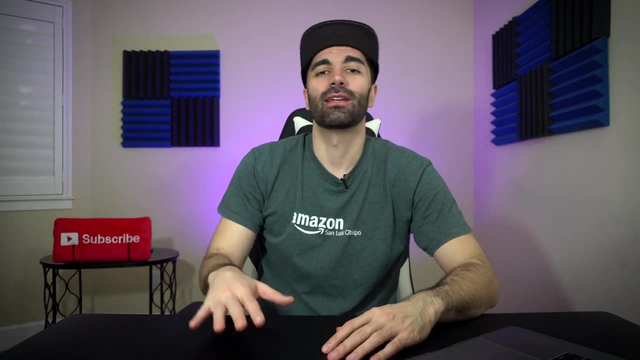 see like if this was impossible. so yeah, I mean, you know, I think you guys so much for watching. you know, go ahead and hit the like button if you enjoyed the video. please leave a comment down below. tell me, you know, is this a strategy that you would consider doing. but, as always, thank you guys so much for watching and have a great day.